80 kiloelectron volts. Now that's a speed of 3,900 kilometers per second. In subsequent years, bigger cyclotrons were built with ever-increasing energies. But how do they actually work Now? the cyclotron basically needs two components. The first component involves this hollow disk. 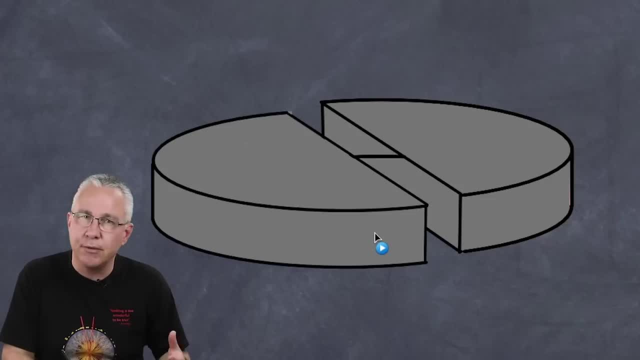 which is separated out, and these two components are often referred to as the Ds, And we have this two Ds. Now what we can do is apply a voltage across them. So in other words, we can have, let's say, one side being positively charged, the other one side being negatively charged. 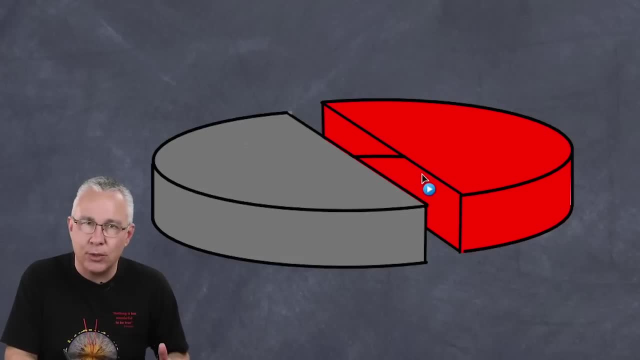 or we could reverse that like so. Now, what does that do? Well, that sets up an electric field between these two Ds, And if I place a charge in between those two Ds, that charge is going to experience a force, it's going to accelerate, it's going to gain in energy, particularly because 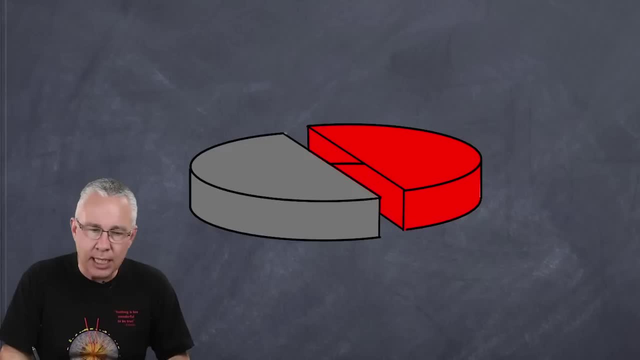 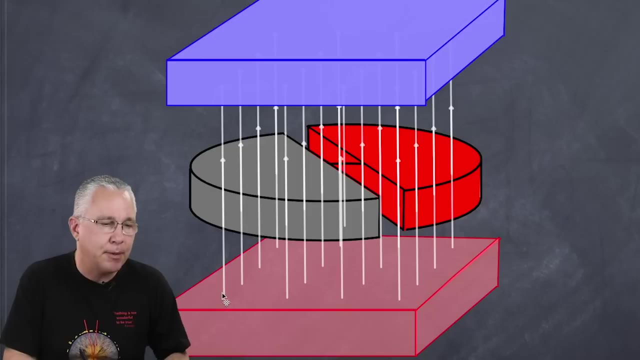 it's gaining in velocity, And that's the key that we want to talk about. The second component is the application of a magnetic field. In this case, the magnetic field is going up the page, And so when we have a charge that is moving within this sphere, it now experiences a force. 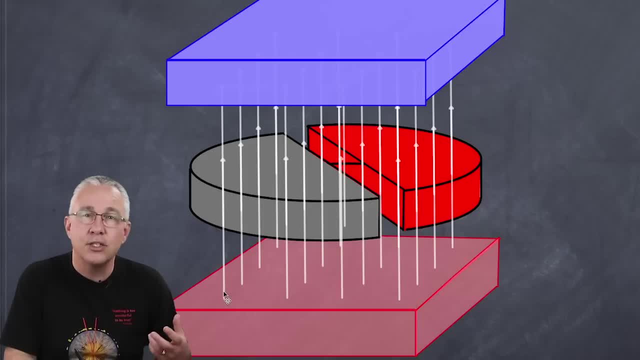 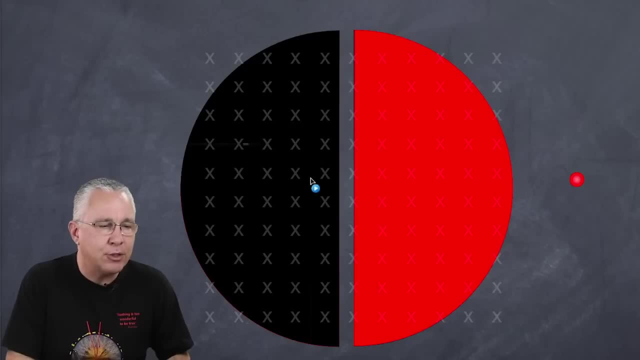 due to the magnetic field, But in this case it experiences a centripetal force. Now to explore that more closely, let's have a look at it from a two-dimensional perspective. So here I have my two Ds and you can see I have a negative side on the left and the positive on the other side, And 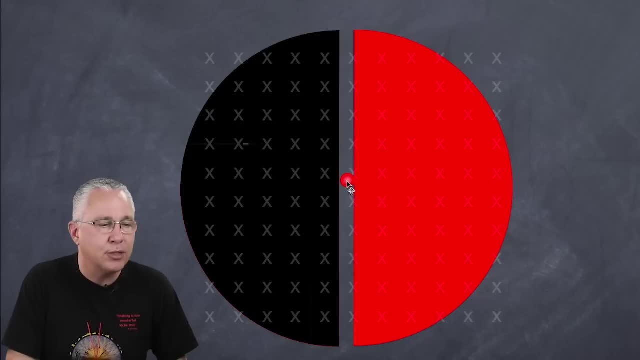 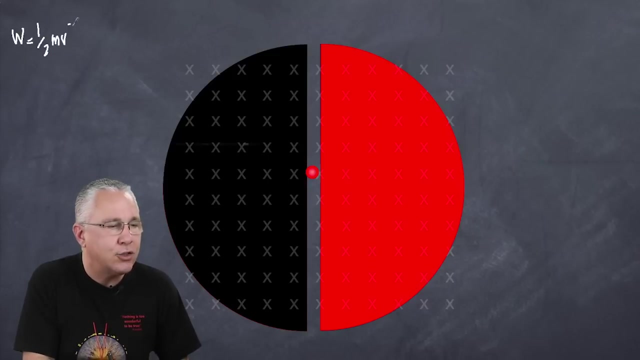 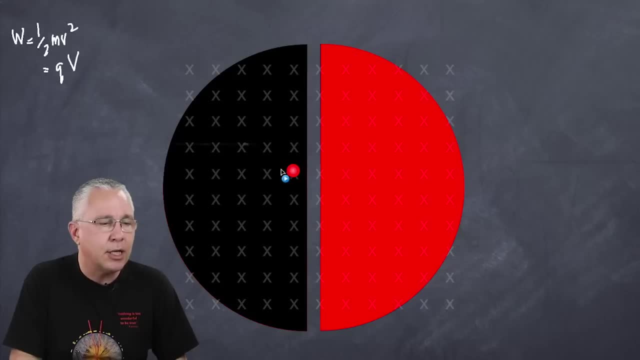 between two differences of potential, and so, in this case, the force that it experiences is due to the magnetic field, but this applies a centripetal force. We know that the Lorentz force is QVB, but this results in a centripetal force which is MV squared over R. Now, if I rearrange this, I'm going to get V over R. 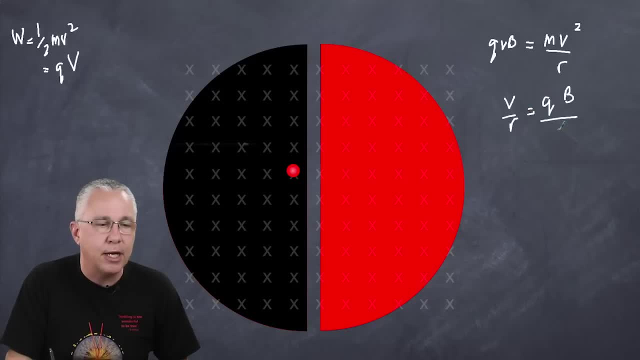 is equal to charge multiplied by B, divided by the mass. In a moment I'm going to explain why I put it in this particular form. Now what's going to happen is my charge is going to now go a circular path with a particular velocity, but then, when it gets to this position here, the polarity changes, and so, as a 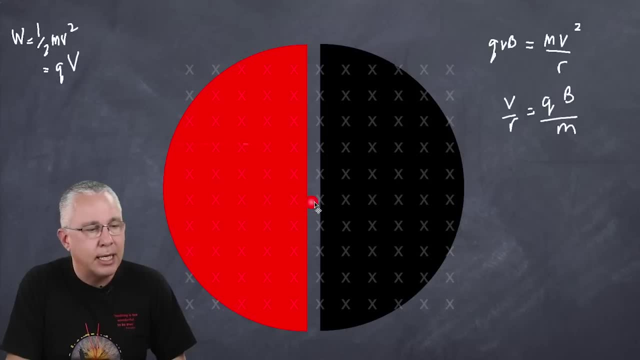 result: it now is attracted towards the negative plate and it speeds up, but now it has an increased velocity. so now it's going to start turn in a large direction. It's going to start a larger arc because it's now moving faster When it gets to. 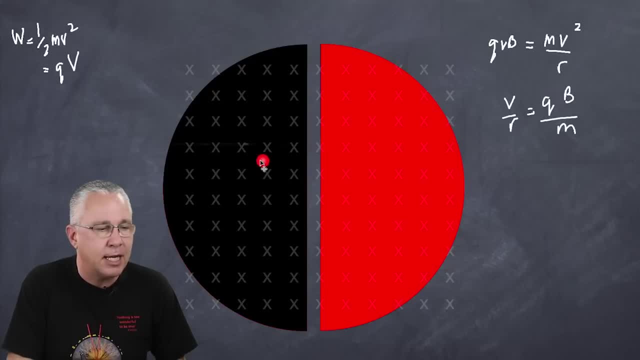 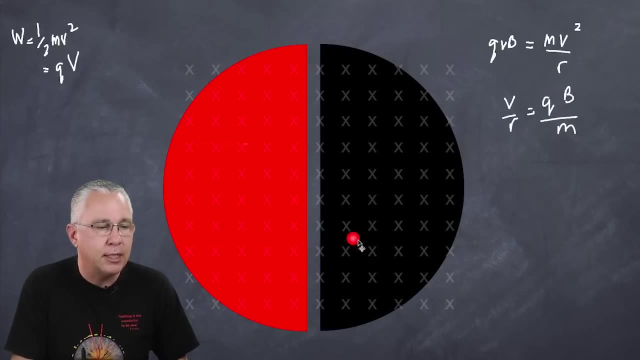 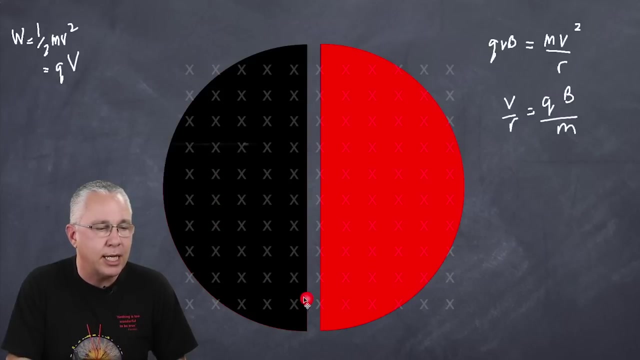 this point over. here the polarity changes, but remember, it's going faster and faster and so, as a result, the radius of turn increases. It gets to here, the polarity changes and the process continues. It goes around and around and continue to go larger and larger and larger every single time, until such time. 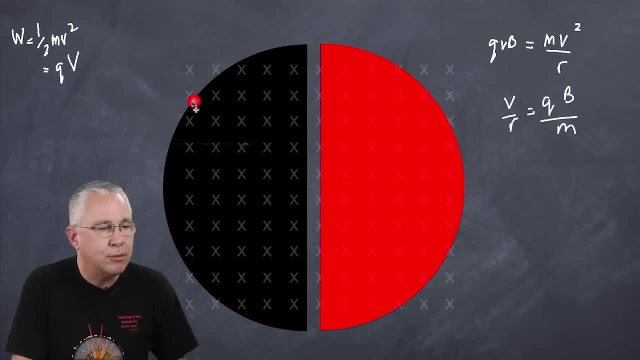 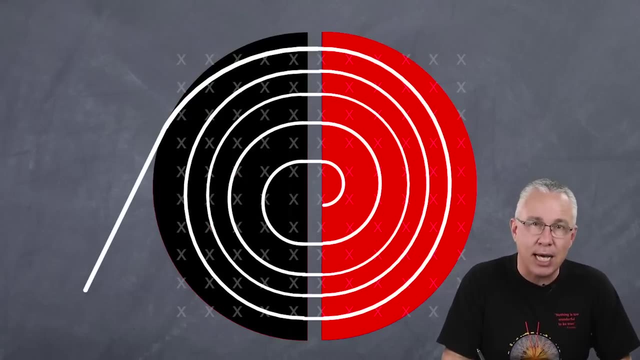 we get to the edge and we may allow the proton to escape, Which means this case it will have a really high velocity. So this is what it looks like. So, in essence, the charged particle spirals out of the cyclotron as it continues to go faster and faster and faster, at a greater and greater radius. 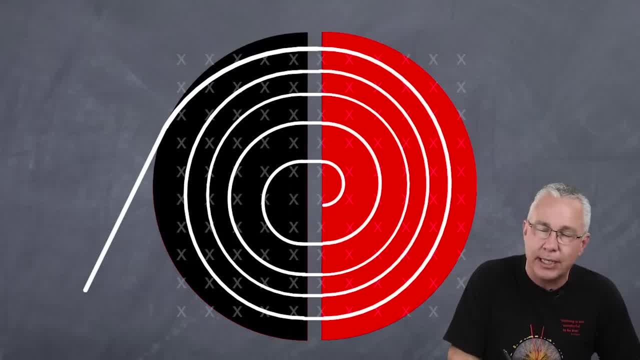 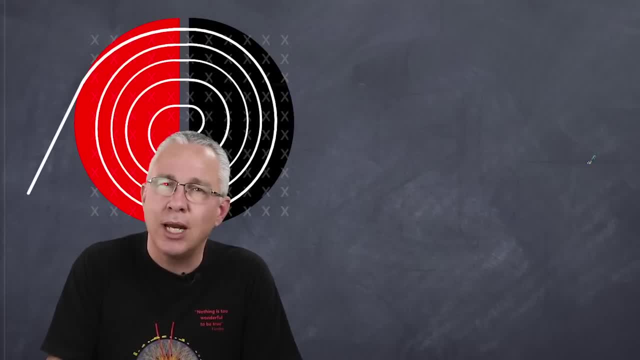 every single time it passes through the D, because of the change in polarity, it continues to increase in velocity. So now we come to the point as to how often does this polarity have to change? What's the rate of change of that polarity? And that is related to the velocity of our proton, In this case our angular velocity. 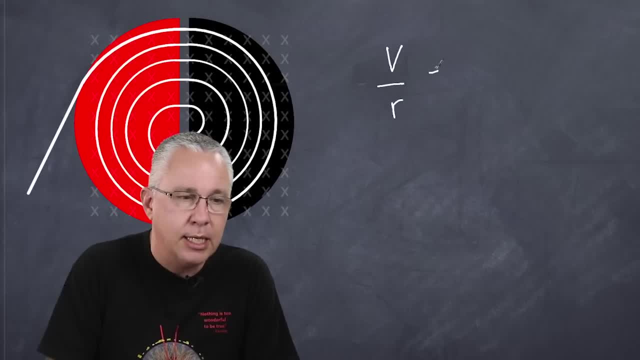 Let me explain. We have a formula which was V over R is equal to QB over M. But if you know your angular velocity formula, which says that the velocity is equal to R times Omega, Omega being the angular velocity, Then V over R equals: 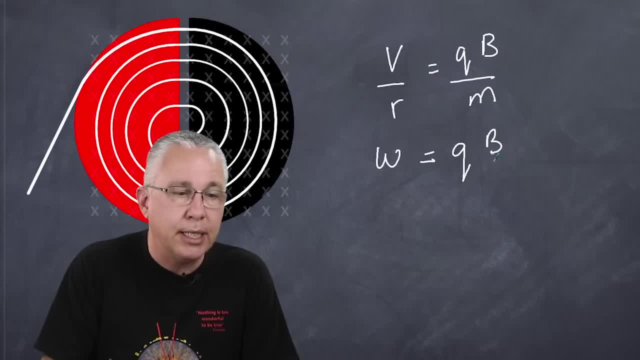 the angular velocity. So angular velocity is QB over M. Now this is rotating faster and faster, faster, in a linear sense, but the angular velocity actually doesn't change. Why? Because the charge doesn't change, The magnetic field doesn't change and the mass doesn't change, So the angular velocity of our proton remains. 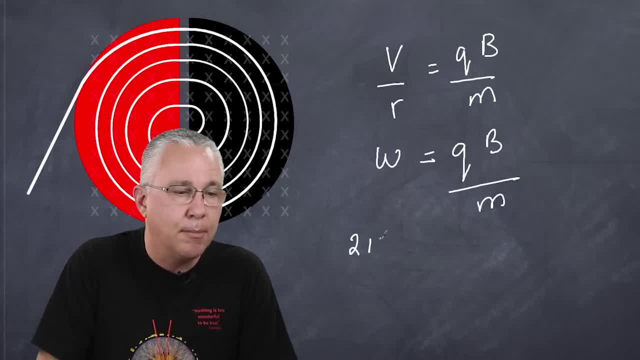 constant, The angular velocity is equal to 2 pi F, which is the frequency of the rotation. So now we get this formula and then we get: the frequency is equal to QB over M. So that's equal to QB over 2 pi multiplied by our mass. That means the frequency of 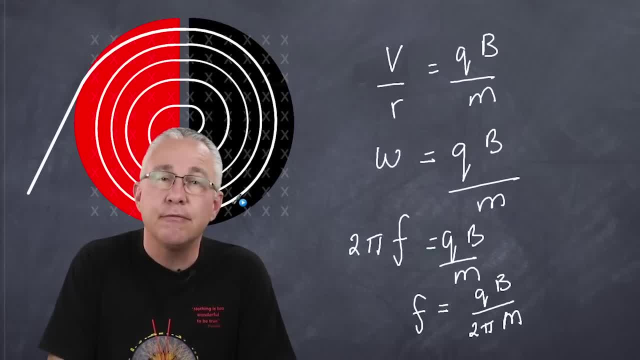 this changing of the voltage has to be the frequency of the charge going across here, And so that's in essence what happens. The voltage changes every half of the period as it goes along, So the frequency of the potential change is equal to the frequency of our charge. 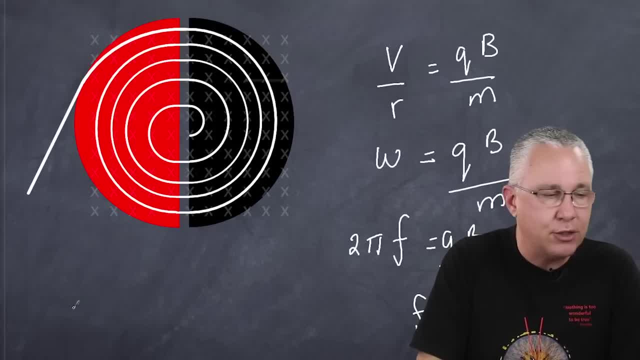 particle And in essence, the voltage is a step function. So in other words, the voltage will look something like this: A positive and a negative voltage, and so forth. And this here is our one period and of course one over that period will give us the frequency of the voltage And that 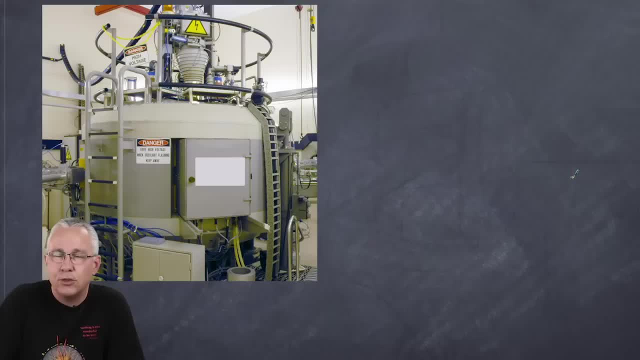 will cause the charge to turn around. So let's apply that to Ensto's, a cyclotron in Sydney. So what do we do? Well, we're going to xy – by the way, we're not going to be using the xy – but we're going to be using the xy – this is an ultraviolet process. So now we're going to take the xy and we're going to say m, v square, So it gets calculated. We're going to get the energy of the particle to be 18 mega and that's 18 mega electron volts. So this is our 11 mega electron volts. 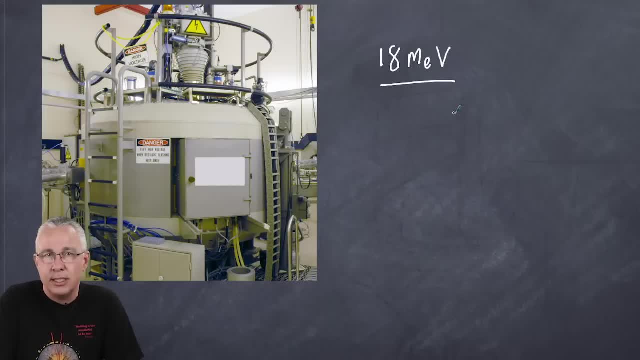 Now, 18 mega electron volts is the energy of our particle. This is the energy of our proton. If we wanted to work out what the velocity is, it's simply a very simple formula, and that is: e is equal to one half m v squared. Now our energy is 18 by 10, to the power of 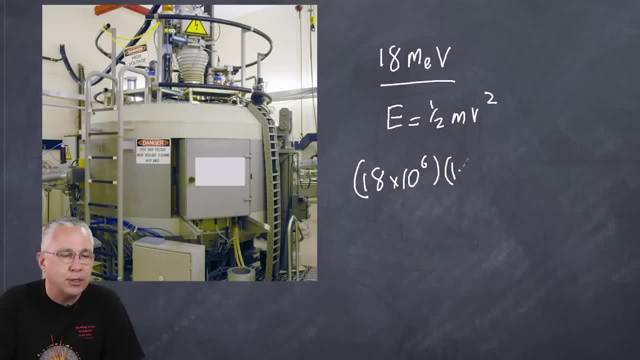 6 electron volts. In order to convert that to Joule's, we multiply it by 1.6 by 10 to the negative 19. 19.. That is equal to half multiplied by my mass of my proton, which is 1.67 by 10 to the power of 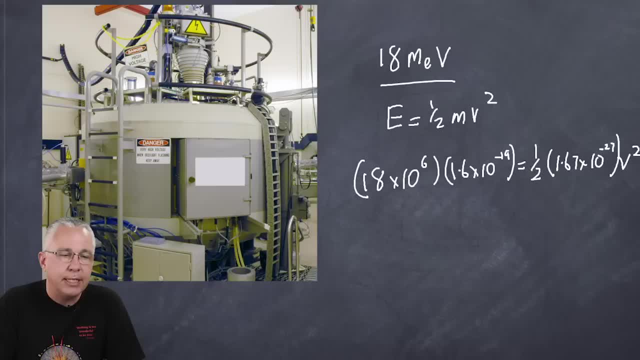 negative 27. multiplied by v squared, The velocity ends up being 5.87 by 10 to the power of 7 meters per second. That is approximately 0.196 multiplied by the speed of light. Now that velocity is reasonably slow, so that any relativistic momentum increases aren't playing. 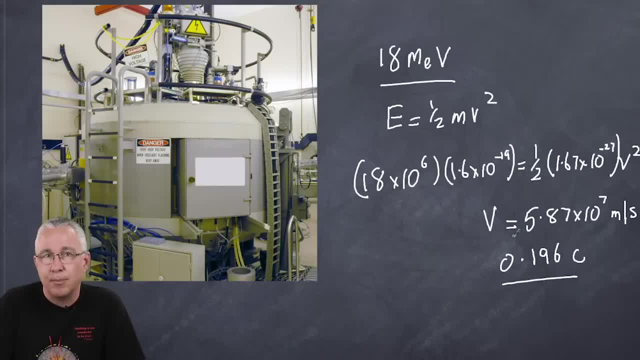 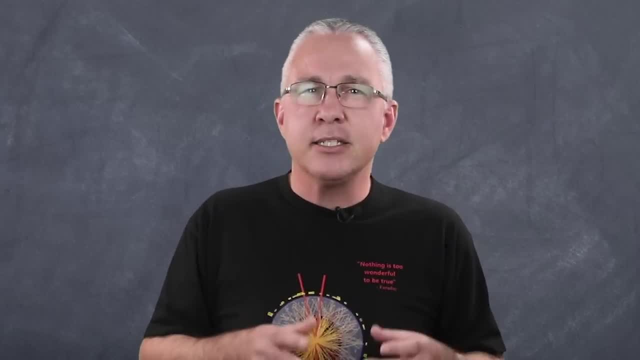 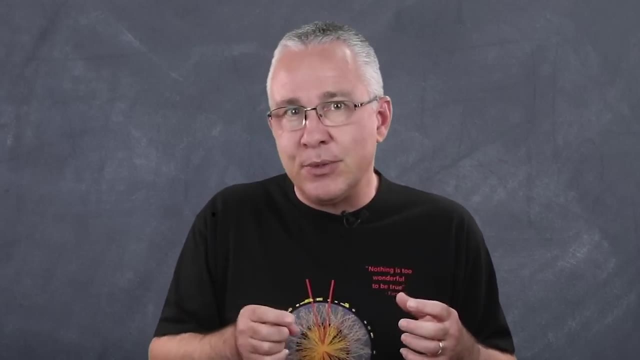 a significant part in the energy of our protons as they leave. But what if you start to get speeds where relativistic momentum is a factor? In essence, the frequency of the voltage has to increase as the momentum increases due to this relativistic nature, and the voltage frequency has to be in sync. 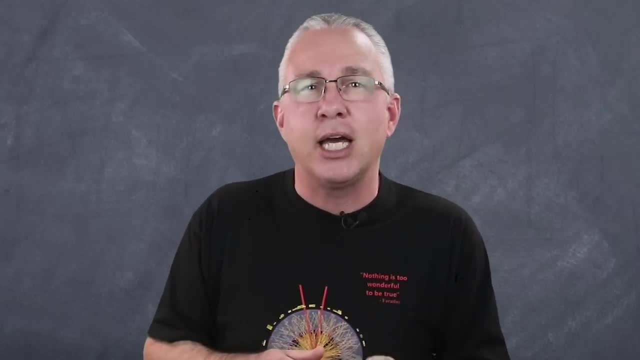 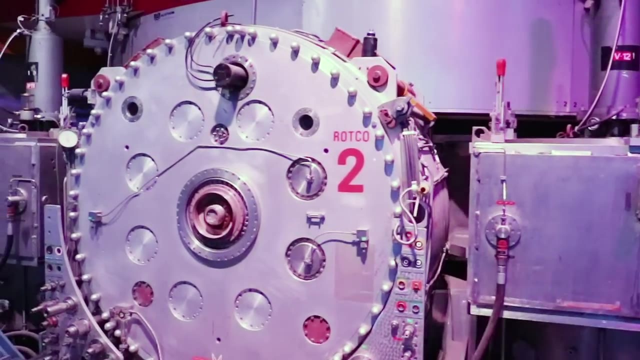 with the rotational velocity. Now that's a much greater engineering challenge, but it's not a big deal. But it led to the development of what is called the synchro cyclotron, which includes the one that was built at CERN in the early 50s. that was CERN's first particle. 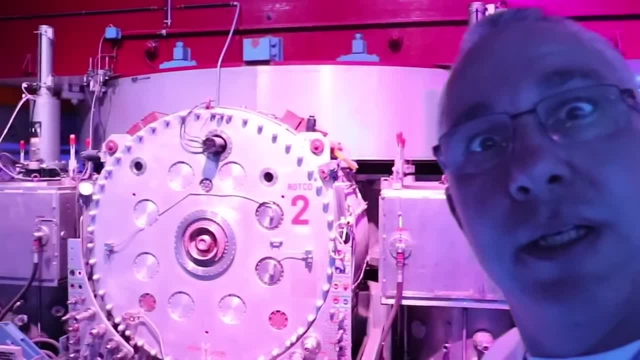 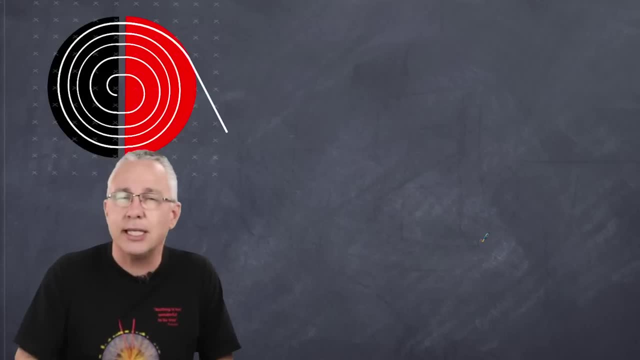 accelerator. And we are here at the first particle accelerator at CERN, the synchro cyclotron. Pretty exciting. So now let's get into the application of our cyclotron. and in the case of anthocyclotron, it produces a chemical called FDG. Now, FDG is a form of a radioactive glucose. 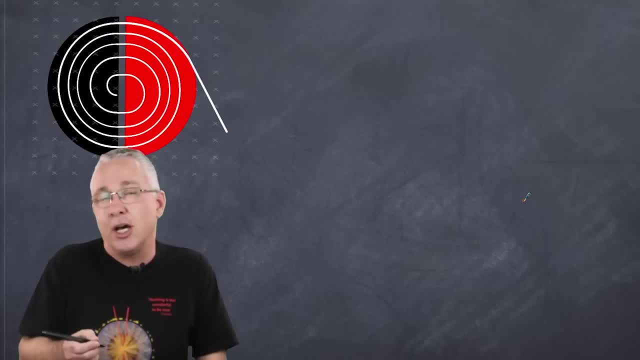 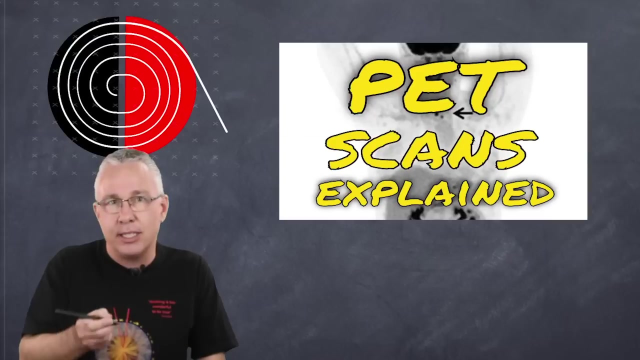 that releases positrons, and those positrons are annihilated with electrons to produce gamma radiation. And wherever glucose is metabolized, this metabolizes, and so you can determine where there is more glucose metabolism occurring by this emission of positrons and the gamma radiation. Now I discuss that further in my videos on PET scans, so check that out if you want more detail. 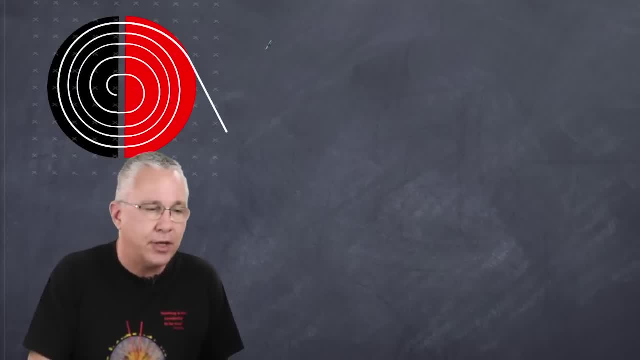 Now, in essence, what happens is that the cyclotron accelerates hydride ions. Now, what are hydride ions? Hydride ions are basically hydrogen ions. So hydrogen ions are basically hydrogen ions that are hydrogen atoms with an extra electron. This is what is accelerated in our cyclotron. Then, as they 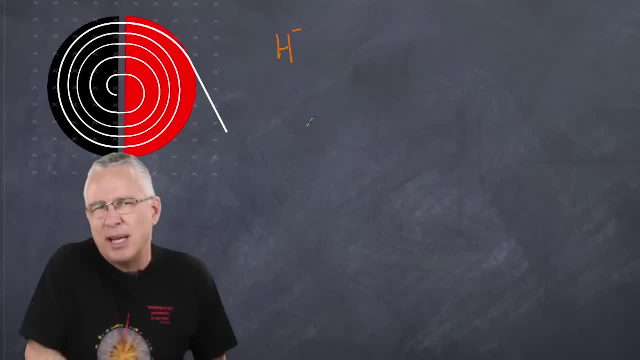 leave the cyclotron, they are passed through as what is known as an electron stripper Basically strips the electrons off it, and so what you end up getting is a stream of protons, because, basically, hydrogen is simply a proton in terms of its nucleus. Now this proton is fired into water. 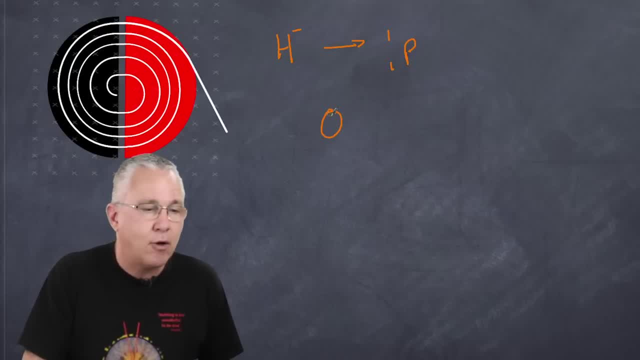 which is enriched with oxygen 18. So we have oxygen 18. It encounters our protons, which are brilliantly well- prévented by hydrogen, and so it triggers their kammination, and that is what we call a fluorescent ion. Now, in this case, the fluorine is being passed.